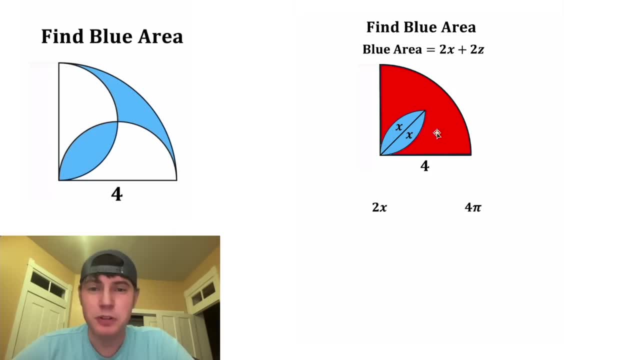 pi And this four pi is the same thing as two of these x's plus two of the y's plus two of the z's. Next, we can divide everything by two On the left-hand side. all these twos will cancel each. 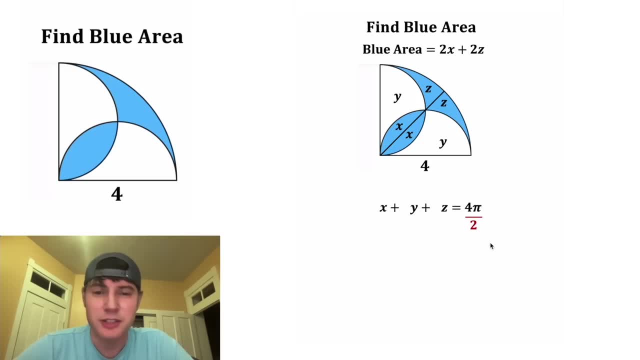 other out And on the right-hand side, four pi divided by two is the same thing as two pi. And then next let's focus on this semicircle, Let's color it red and let's find the area of the red. The area of a semicircle is pi r squared divided by two. This four is the. 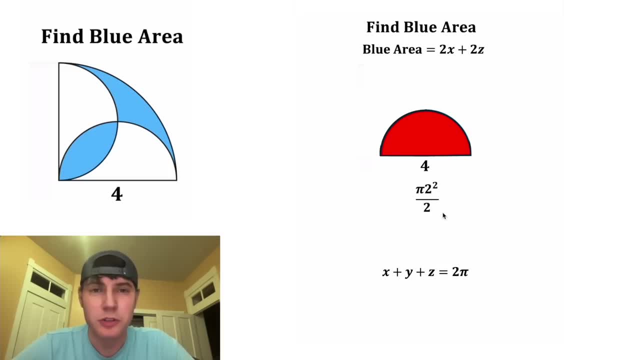 diameter of the semicircle, which means the radius would be equal to two, And two squared is equal to two times two, and these twos will cancel each other out. So the area of this red region is equal to two pi, And this two pi is the same thing as 1x, 2x plus y, And now we can bring everything. 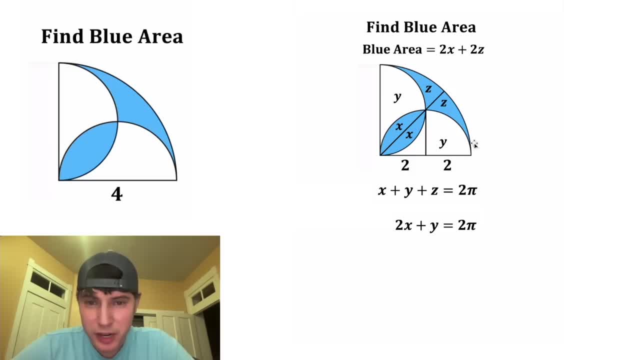 This four would split into two by two, and then this radius wraps all the way around, so this height is also two. Now let's focus on this quarter circle. This x piece plus the triangle will equal the whole quarter circle. Next we can subtract triangle from both sides. These triangles, 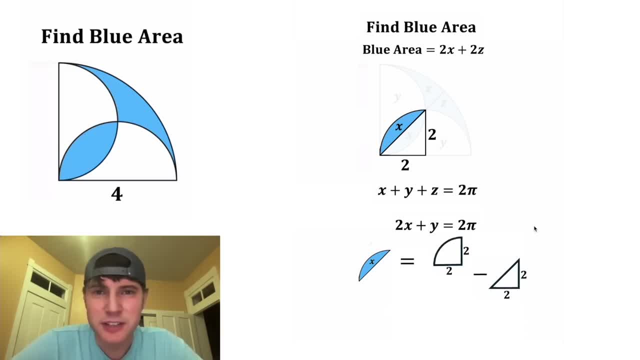 will cancel each other out. On the left-hand side we'll have x and on the right-hand side we'll have quarter circle minus triangle. The quarter circle, which is pi r squared, divided by four. The triangle, which is base times height divided by two. The radius of this quarter circle. 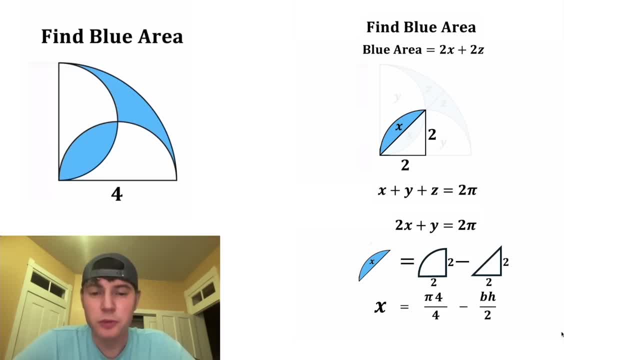 is equal to two. And then on the left-hand side we'll have x, and on the right-hand side two squared is equal to four, and these fours will cancel each other out. So the quarter circle has an area of pi, And then for the triangle the base is equal to two and the height is equal to. 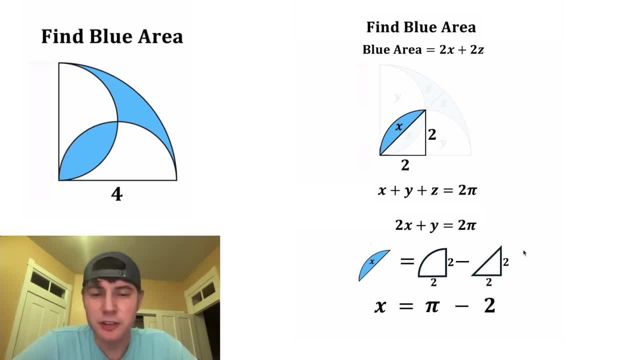 two. These twos will cancel each other out. so the area of this triangle is equal to two. And now we know that x is equal to pi minus two. In the place of this x, we can plug in pi minus two, This two. 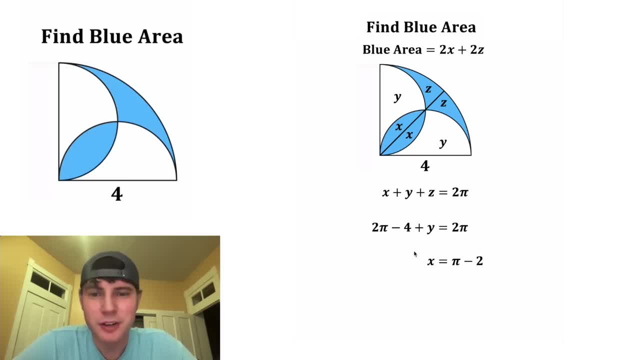 is going to distribute to both of these. so it becomes two pi minus four. Next, let's subtract two pi from both sides and let's add four to both sides. On the left-hand side, these two pi's will cancel each other out. These two fours will cancel each other out. And on the right-hand, 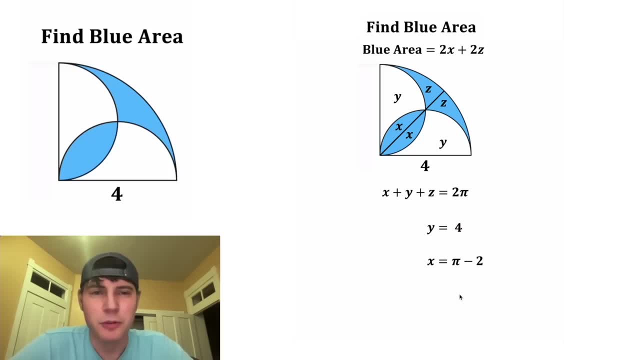 side, these two pi's will cancel each other out. so we have y is equal to four. Now we know x and y, so we're going to substitute that into this equation. In the place of the x we'll plug in pi minus two, And in the place of the y we're going to plug in four. Let's combine the negative.